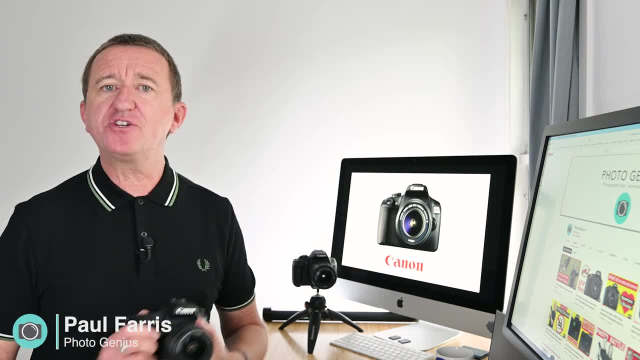 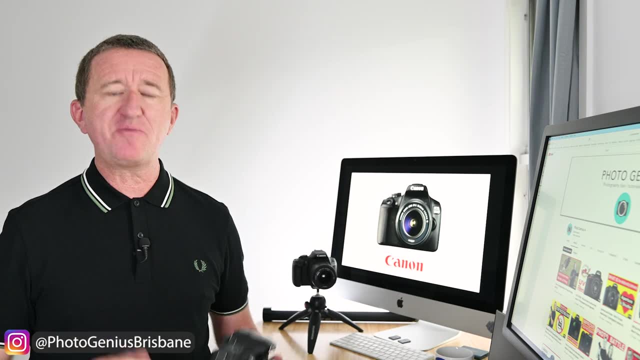 If you are new to the channel, please consider subscribing so you don't miss out on future videos. Now, generally speaking, when most people get a brand new camera, they start off by using the camera in the auto mode, which, of course, is fair. The camera is making decisions on your behalf, and this means you can't be creative with your camera. 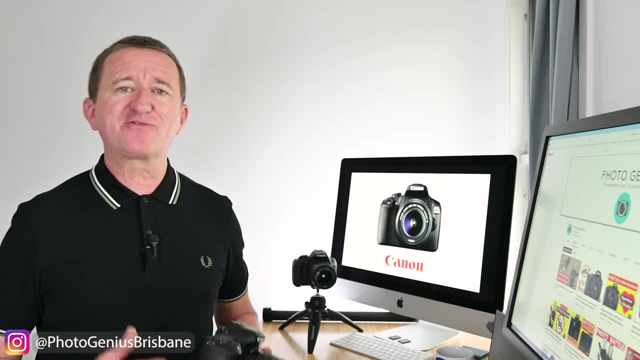 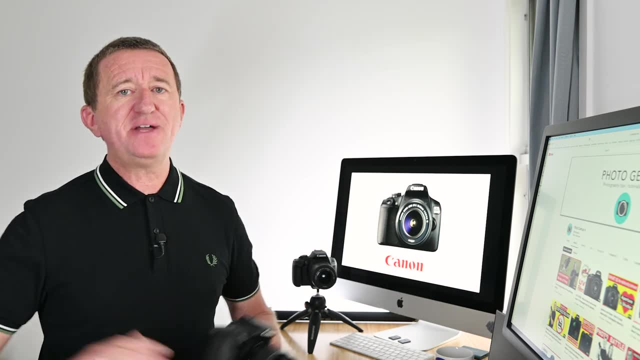 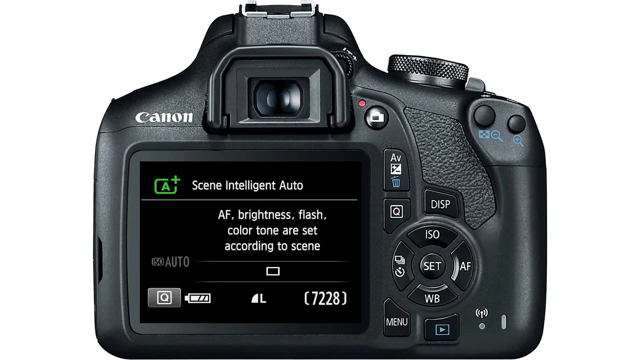 So if you want to get more from your camera, take better photos and, of course, be more creative, at some point you're going to want to get out of auto and start exploring the manual modes, And that's what this channel is all about. So let's take a look at the LCD screen on the back of a typical Canon EOS camera. 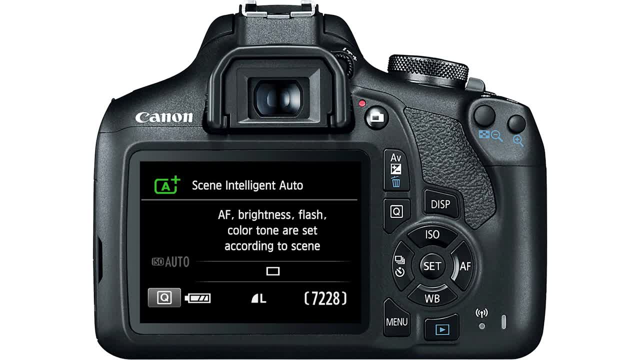 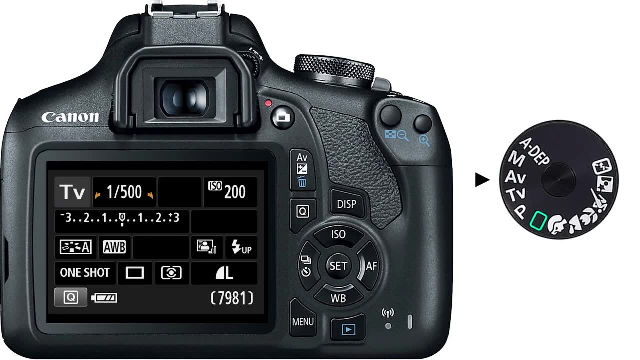 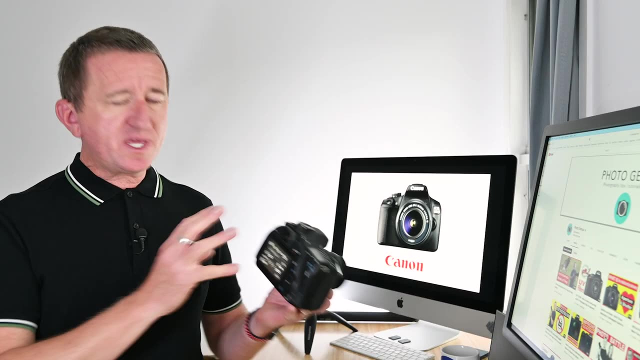 With the camera set to auto, the info displayed is very clear. It's fairly limited, but if I change the camera mode to program shutter priority, aperture priority or manual, you will see a big change. Now, as a beginner, all the information displayed on this screen can be really confusing and 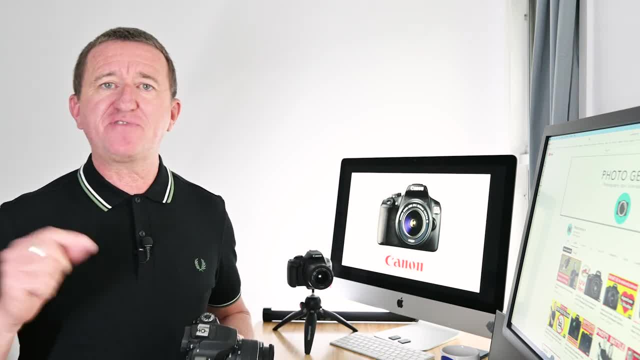 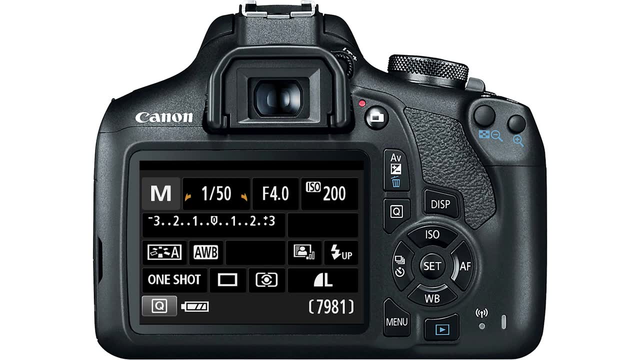 overwhelming to begin with, but don't worry, because the cameras feature guide that is built into most Canon cameras is there to help. Let me show you how it works Now. to begin with, the feature guide is currently turned off. Now let's say I want to find out more about what AWB means. 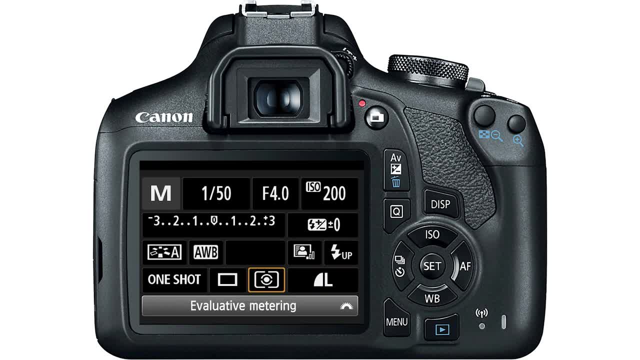 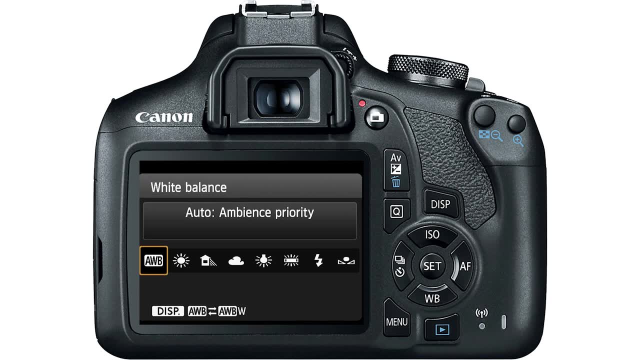 I press the Q button on the back of the camera, I select AWB and press set. Now we can see that this is the white balance function And as I scroll along the different icons, we see there are lots of options, But the camera doesn't tell me why or when I may wish to use these. 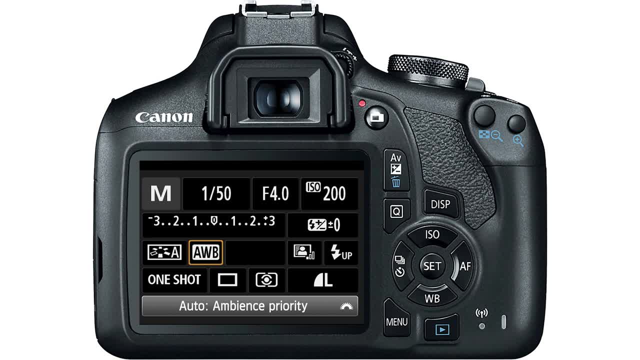 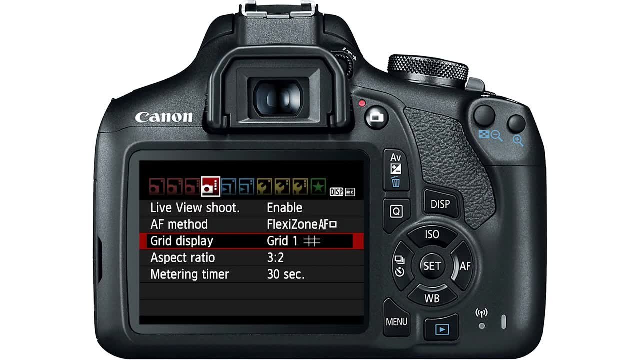 So for now I'm going to go back to AWB Press set once again, And now I'm going to turn on the guide mode. To do this, I press the menu button, I select yellow custom menu number two. I then scroll down to feature guide and of course I'm going to change this to enable 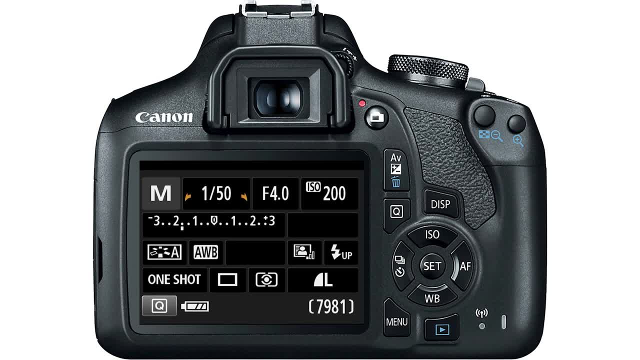 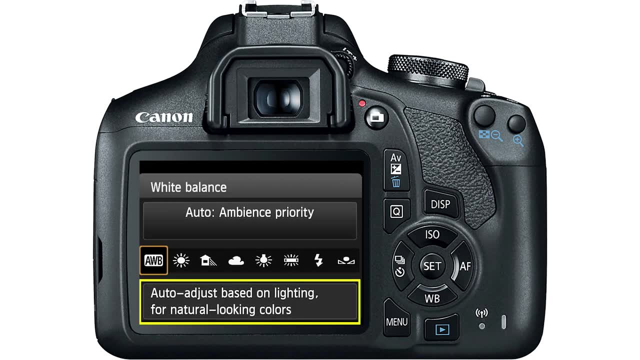 Now let's take another look at white balance. Again, pressing the Q button, I select AWB and this time we see that we have an info panel at the bottom of the screen and this shows me that white balance will automatically be adjusted to help give my images natural looking colors.